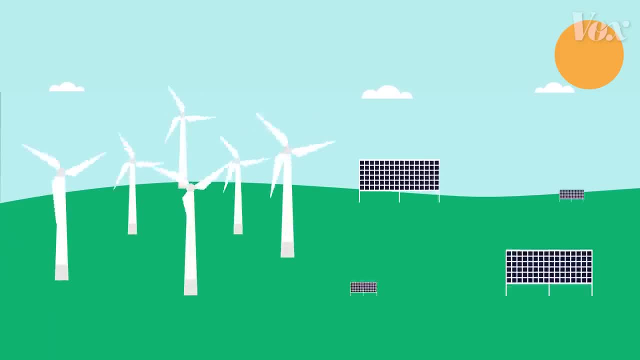 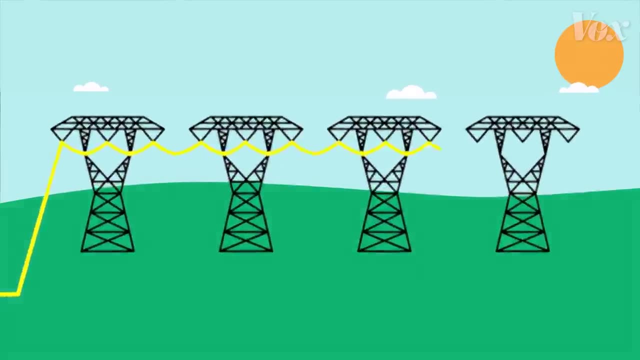 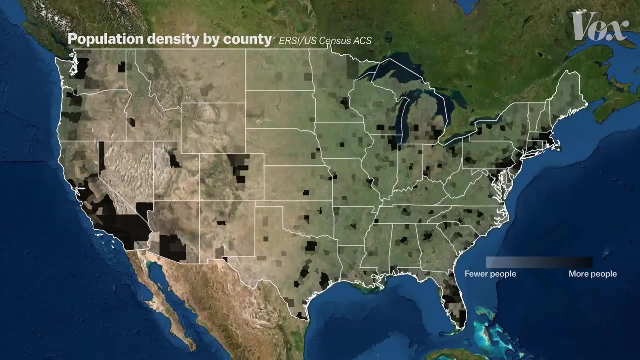 If we want a greener future in the US, we'll need to build more renewable energy plants. But to actually use that electricity, we'll also need to build more of these. This is a map of where everyone in the continental US lives. 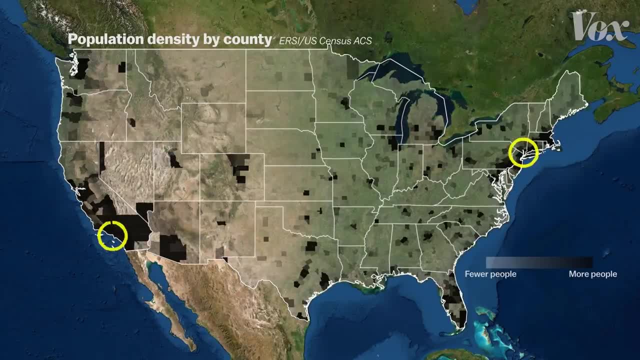 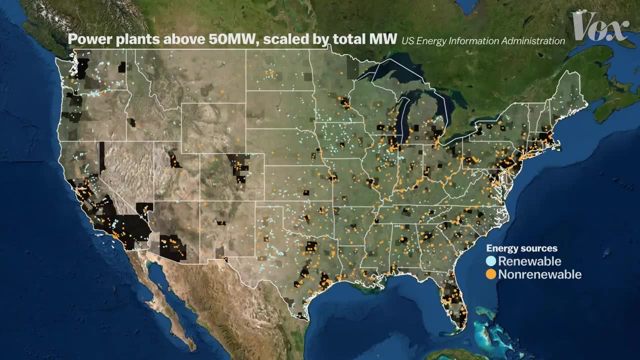 the density of each county. Here's New York City, LA, Chicago, And here's where every big power plant is currently. Appropriately, they tend to be where the people are. In Washington DC, where I live, we get nearly all our electricity. 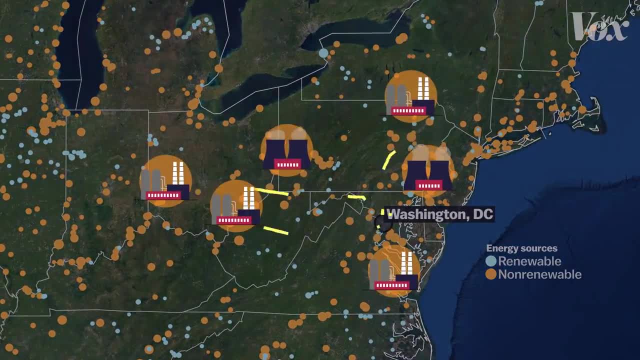 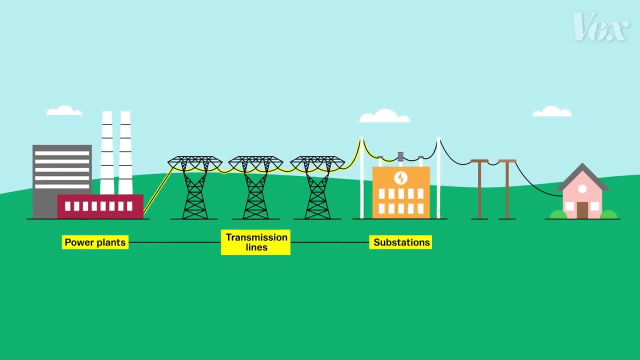 from surrounding states' power plants, mostly nuclear and natural gas. Electricity goes from the power plant through big high-voltage transmission lines to a substation where the electricity is dispersed onto smaller, lower-powered distribution lines that send it into my house. 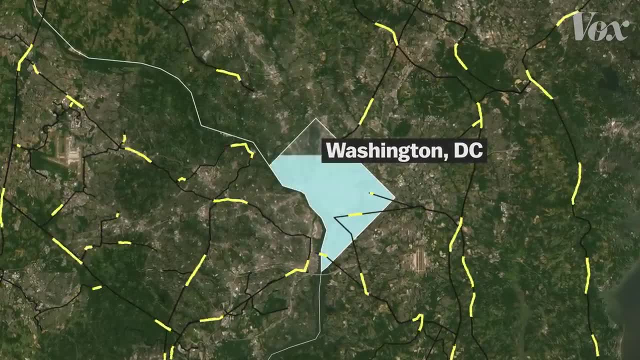 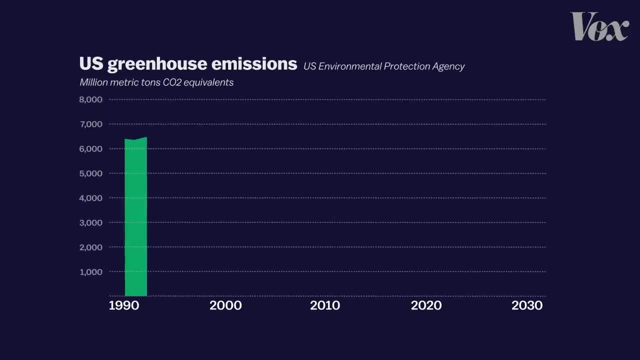 Like Vermont, DC also plans to be greener. The goal is to have 100% renewable sources, making our electricity, by 2032.. It's part of a national goal too. President Biden wants to reduce emissions in the US 50% by 2030, Which is quite a new pace. He's also trying to be prepared for any future upheaval that may be in the way of third-party electricity in the US. It's also part of a national goal too. President Biden wants to reduce emissions in the US 50% by 2030. 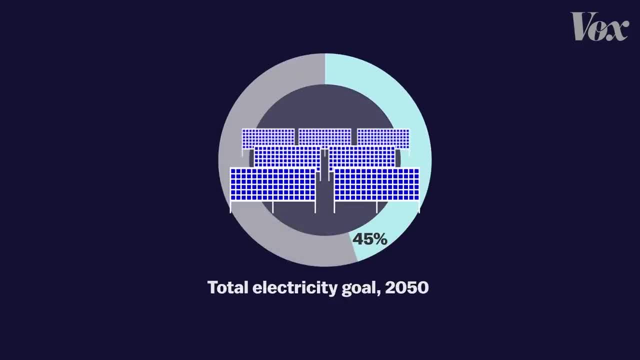 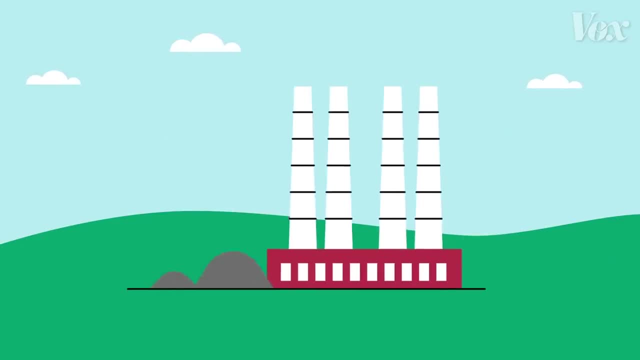 President Biden wants to reduce emissions in the US 50% by 2030.. with nearly half of US power coming from solar plants, by 2050. That means switching out those natural gas plants for wind turbines, coal plants for solar farms. 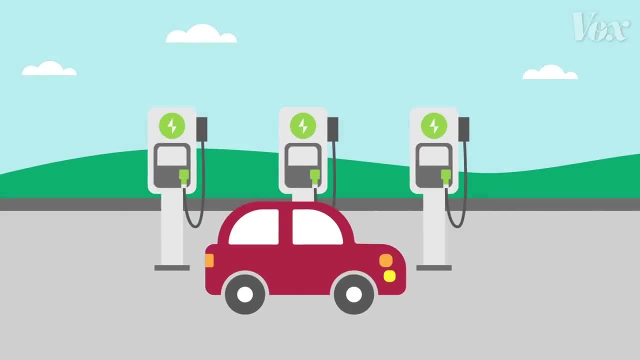 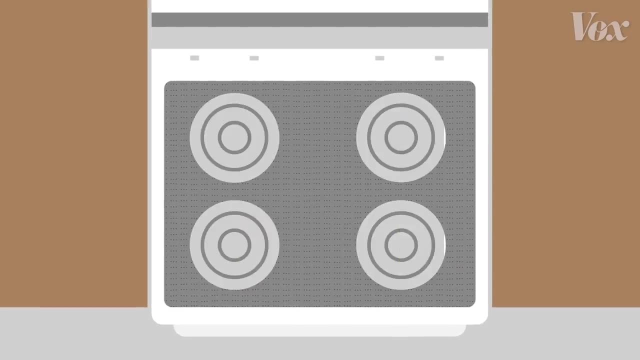 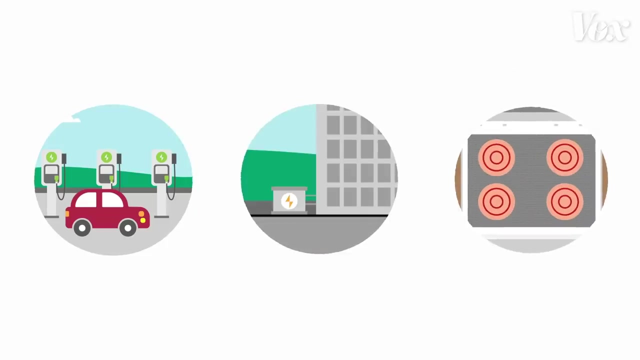 Lowering emissions also means switching from gas cars to electric cars, heating our buildings not with natural gas, but with electric heat pumps, cooking on electric stoves. Basically, we're going to be using a lot more electricity- anywhere from 40% to 100% more than we currently use. 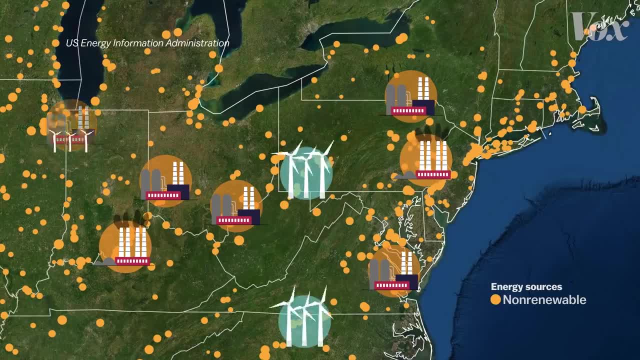 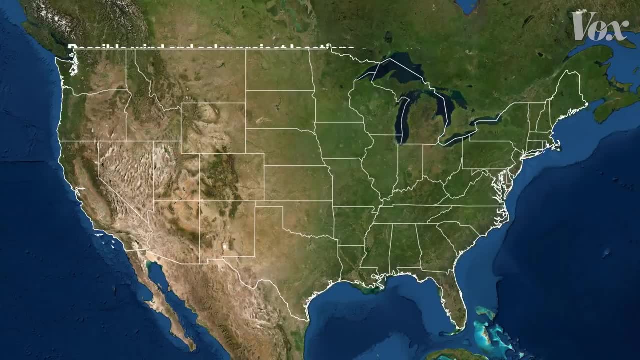 So back to the map. If we're going to replace all these polluting energy plants, we can't just build a wind turbine in their place. They need to be where it's, you know, windy. This is a model created by Princeton. 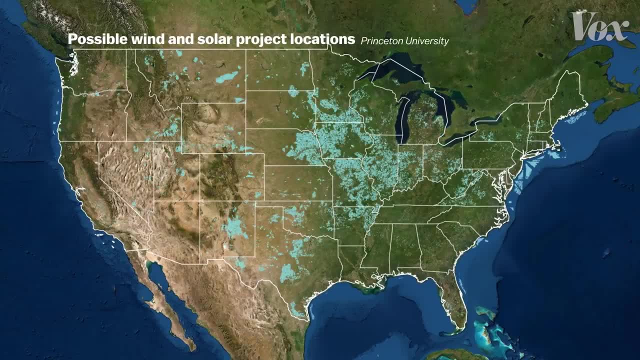 mapping out possible places in the continental US where wind and solar projects could, in theory, be built. Aside from some offshore wind farms, it's mostly in the middle of the US. Another study found that these states have most of the wind and solar potential. 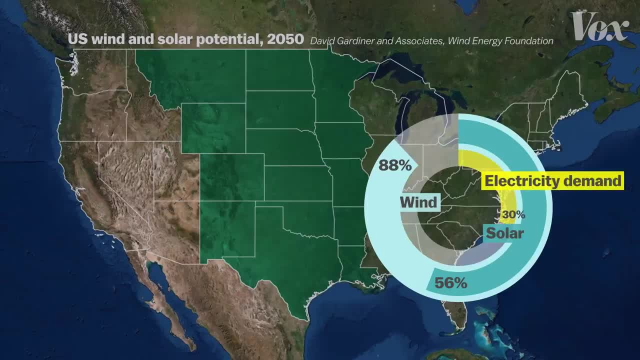 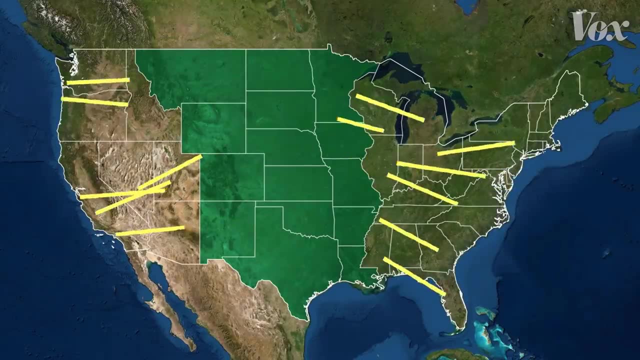 yet the people living there would only make up 30% of the electricity demand. In a decarbonized future, we're going to need to get electricity from here to here And we're going to move a lot of it. That's where high voltage transmission lines come in. 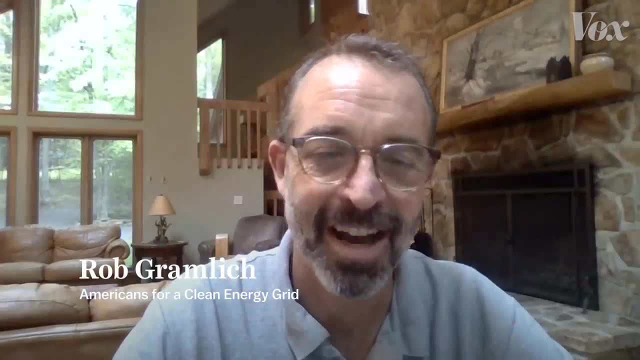 I think the infrastructure is the most important thing. It doesn't get a lot of attention, but it really is the key. This is where the wind and solar power lines come in. This is where the wind and solar power lines come in. This is where the US currently has high-voltage transmission lines. 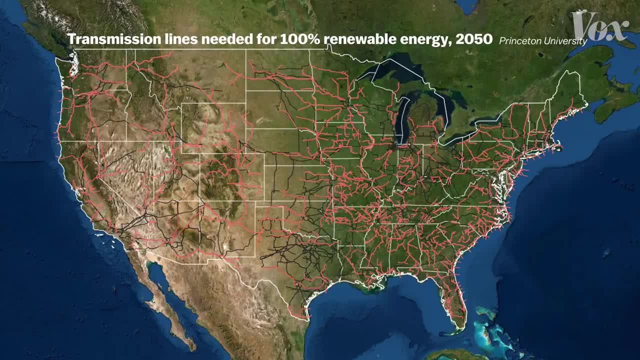 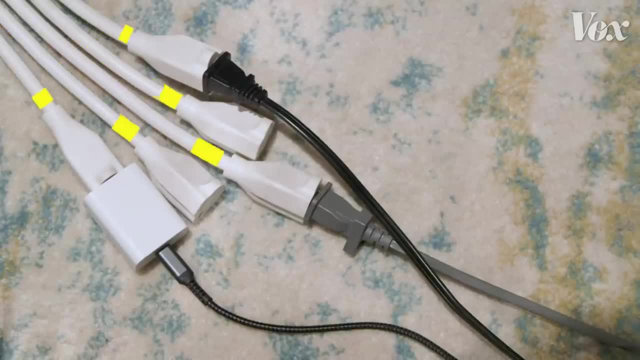 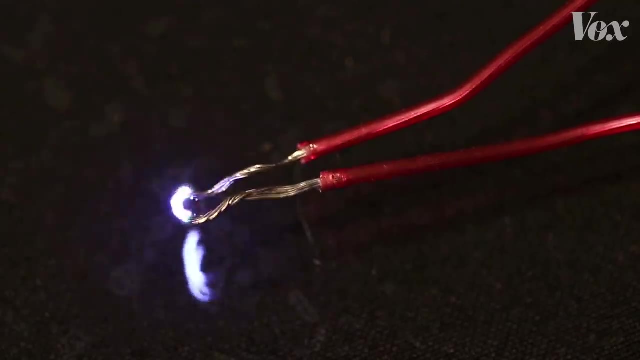 The Princeton model shows us. this is where new lines will need to be built if the US uses all renewable energy by 2050.. But it's not a simple process. Every wire in your house has plastic over it, because if two electrical lines get too close, 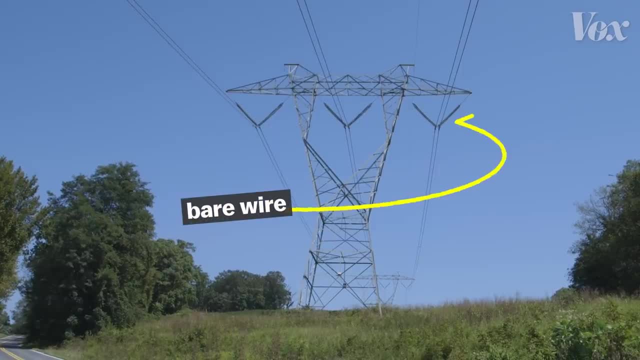 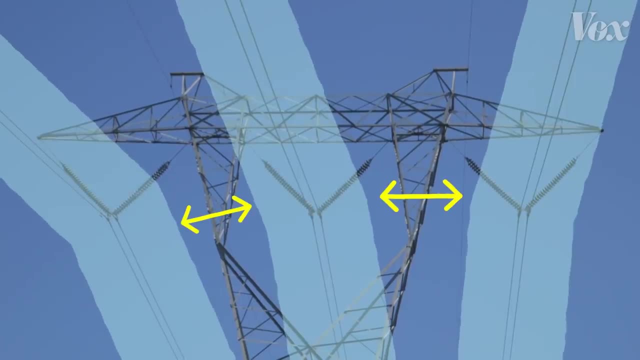 But high-voltage power lines are the bare active wire, No plastic. They're insulated by the air Basically, if they're kept fresh far enough apart from each other, it's safe. But they also have to be kept far away from everything. 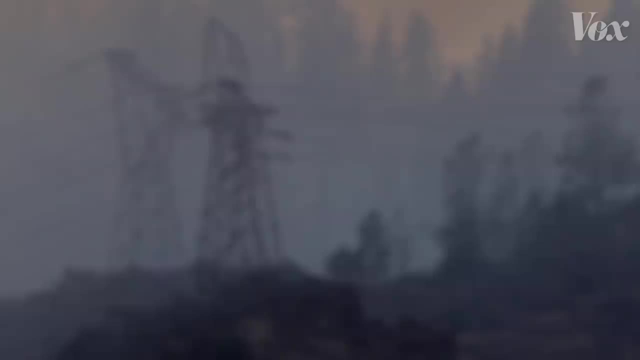 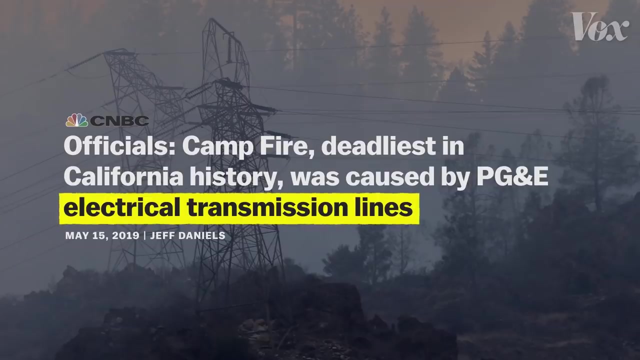 Trees included. This is actually how some of the California wildfires were started: Trees coming in contact with the super-big high-voltage transmission lines, And those are what we'll need more of as we lengthen the distance from energy source to energy need. 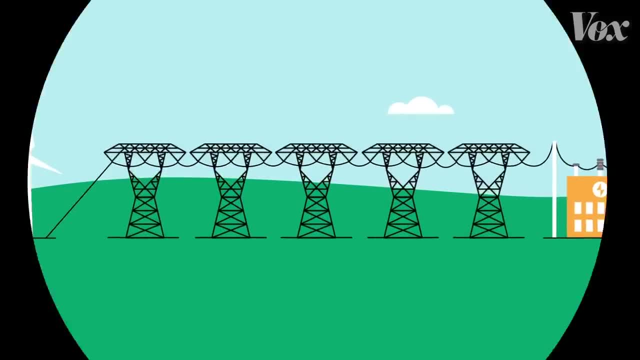 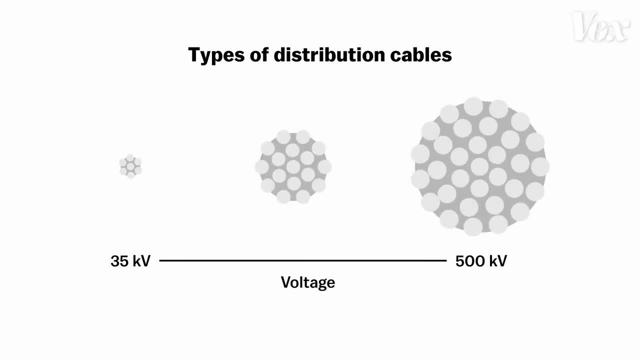 We'll also need to make many current ones even bigger, Because bigger means more power. Physically, the cables are thicker. The bigger the cable, the more power can run through them. And because they're bigger, they have to be really far apart for insulation. 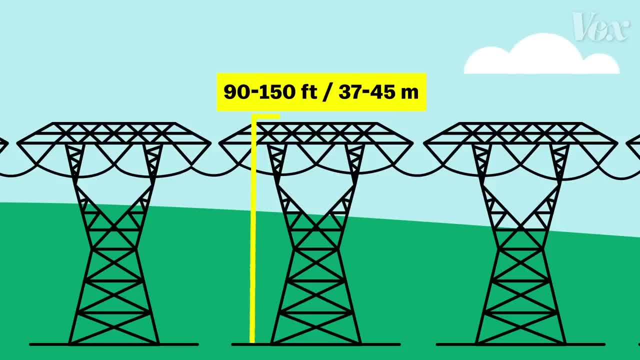 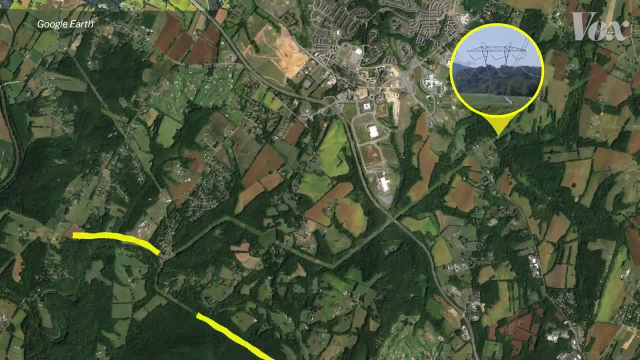 And built higher up. It makes them kind of a pain to build, partly because of how large they are but also how much private land they have to cross. Very often the developer can get 99% of the landowners to agree. 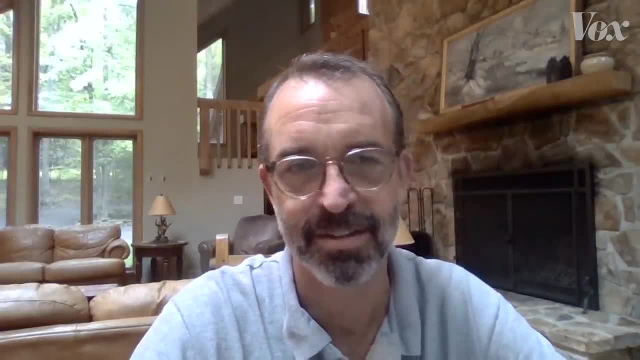 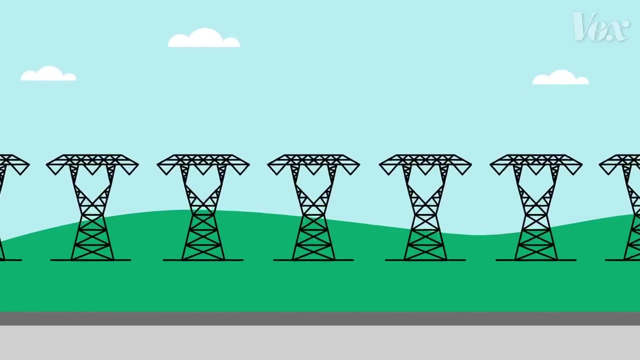 but then there's that last 1% and that can take forever and can crater the whole thing. So experts say we should start building now, even before we build the plants. You can do a generation project in a year, The transmission 3 if you're lucky, but it can go over 10.. We don't want to do this in a reactive mode where we build a lot of stranded generation. We want to proactively build the transmission to where we know the resources are, And the thing about wind and solar resources is: we know where they are.